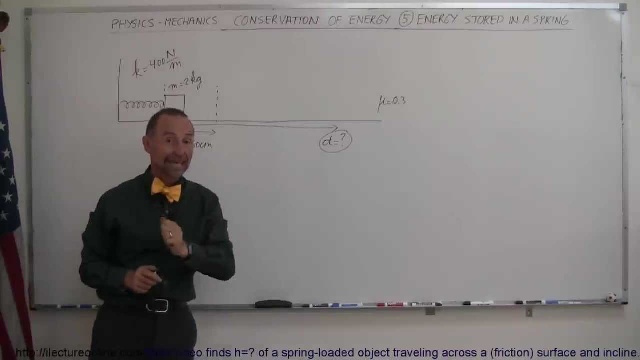 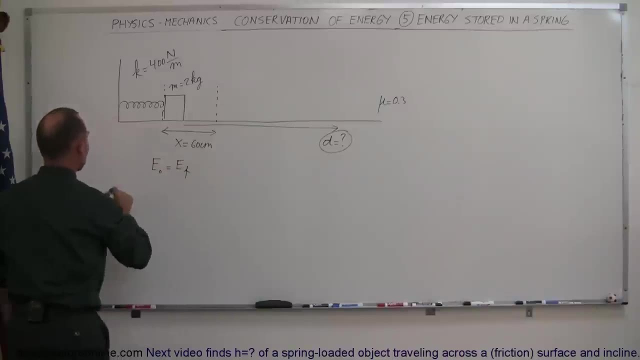 We can simply look at the initial state and the final state and get the correct answer. So let's try that. So we can say energy initial equals energy final, which means that any work put into the system plus the potential energy initial, plus the kinetic energy initial, 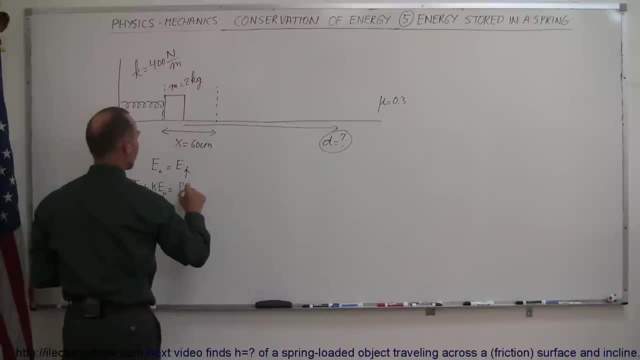 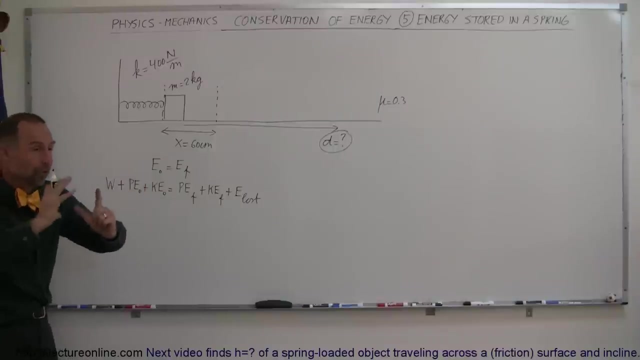 must equal the potential energy final plus the kinetic energy final plus any energy lost by overcoming friction. Now you may say there's work done because we have to compress the spring. Well, either you account for it by the work done to compress the spring. 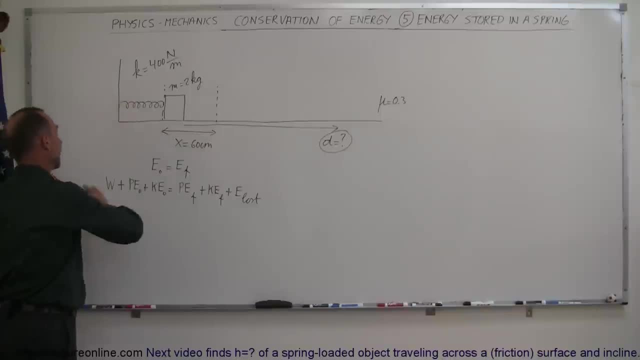 or account for it by the energy already stored in the spring, And then we don't have to take into account the work done. So in this case we could say the work done was done prior to the problem got started. Energy was already stored in the spring, so we don't have to worry about that. 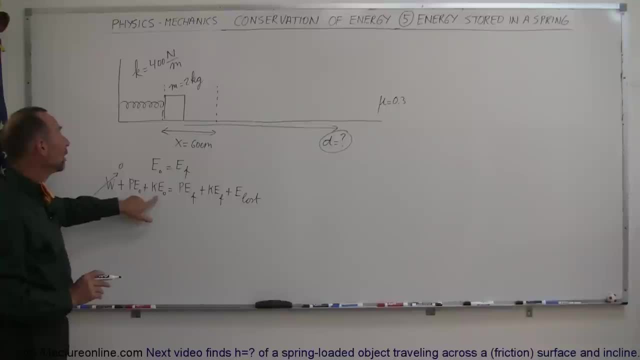 Potential energy stored in the spring. yes, we have No kinetic energy because nothing is moving at the moment. we let go of the block, so zero kinetic energy. There's not going to be any potential energy. final, because there's no altitude gain, no height gain. 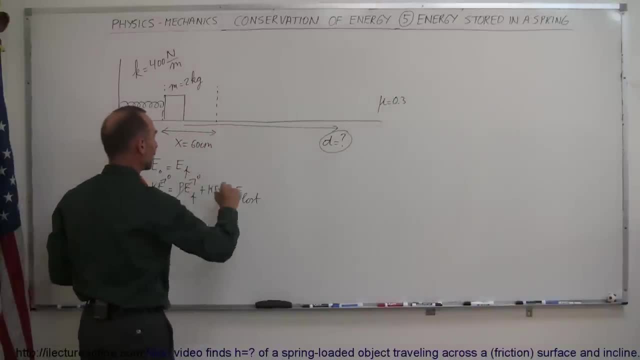 so there's no final potential energy. The block will not be moving at the end, so that's zero kinetic energy. So, really, what happens now is it's a simple equation- where the initial potential energy stored in a compressed spring, well, all of it will be used to overcome the energy lost E lost. 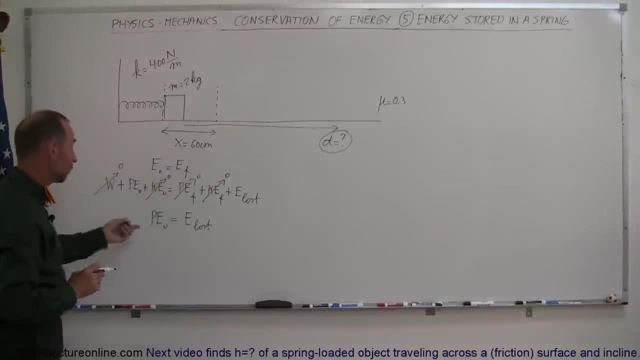 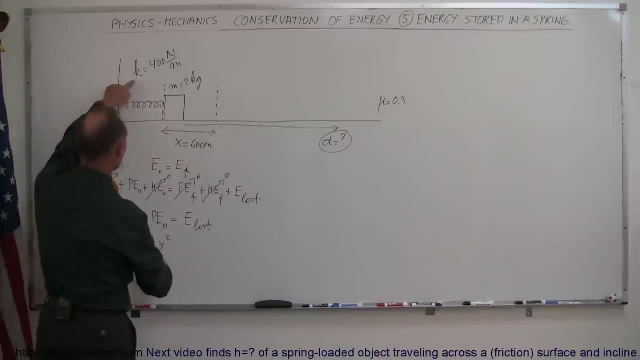 And now we just have to figure out what those things are. For the potential energy initial, the energy stored in the spring, is one-half k, x squared, k being the spring constant and x being the distance that the spring was compressed. Of course we'll have to convert that to meters. 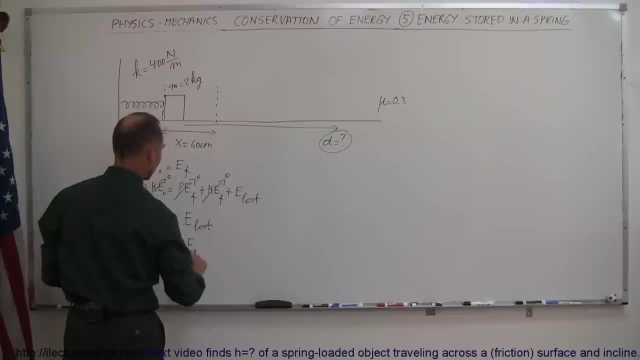 And the energy loss is going to be equal to the, the friction force that we have to overcome times the distance that we have to travel and, of course, that's what we're looking for. That's the variable we're going to be solving. 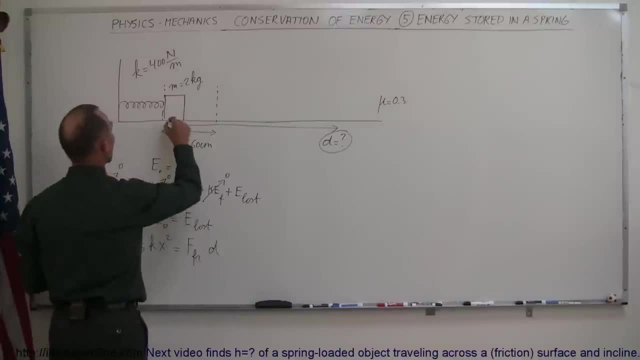 The friction force on a flat surface. remember there's going to be the weight of the block pushing down mg. We're going to have the normal force pushing back from the floor upward, normal force which is equal in magnitude to mg, of course, opposite in direction. 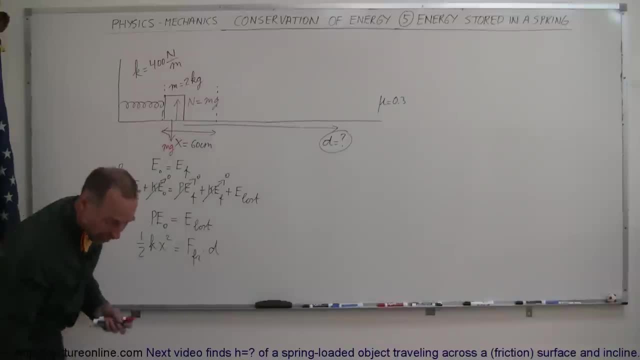 And then the friction force will of course be in the direction opposite of its motion. so the friction force will be in this direction. That will be equal to the normal force times mu. So in this case that's going to be mg mu.